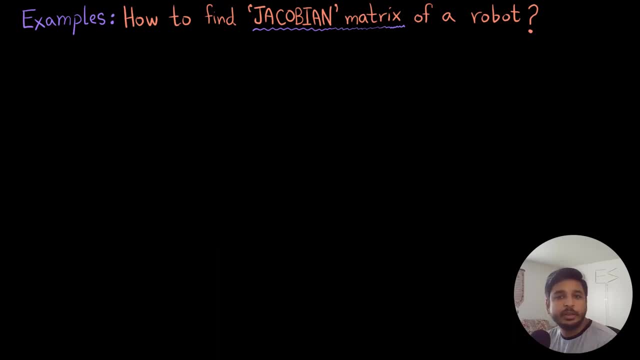 hi everyone, welcome back to another video in this video series on robotics 101. i am zain khan and in this video we are going to talk about how to find the jacobian matrix of a robot. we are going to do a couple of examples together. so for the first example, i have this fancy yellow robot right here. 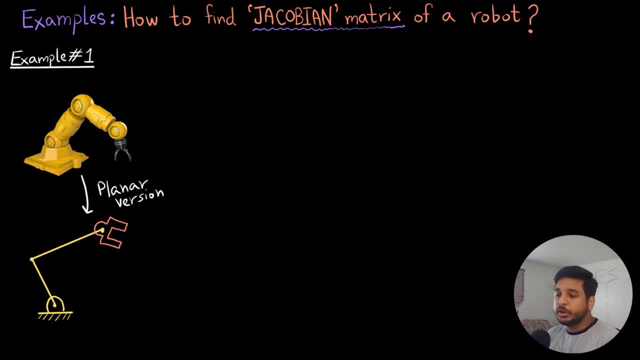 which is a 3d robot and i have converted into a planar version down below, which has got three revolute joints. so it has got three motors attached here, here and here. so it has got three motors. that i at these three points and it can revolve around these three points. now just marking. 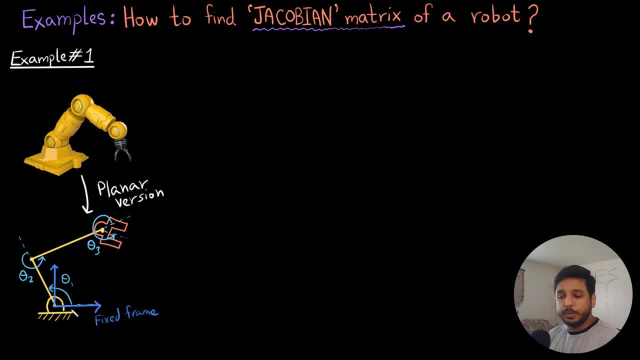 out a few things. so i have marked out the fixed frame in blue and i have marked out the three angles: theta one, theta two and theta three. now, before we go on to finding out the jacobian, i just wanted to bring your attention to a couple of things. firstly, whenever we are talking about the robot's, 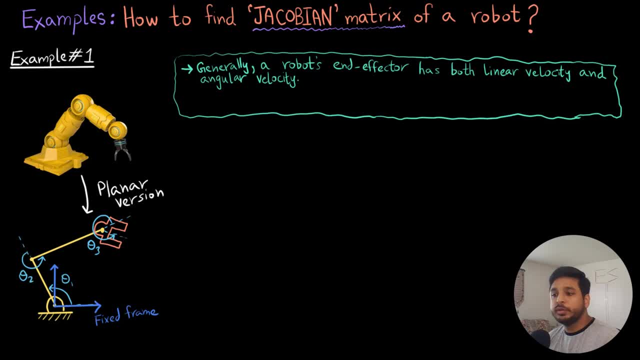 end effector velocity. so we need to keep in mind that the velocity of the end effector is going to comprise of two distinct velocities, the first being the linear velocity, which is just how fast the robot moves in the x and the y direction, and the other is the angular velocity, which is how 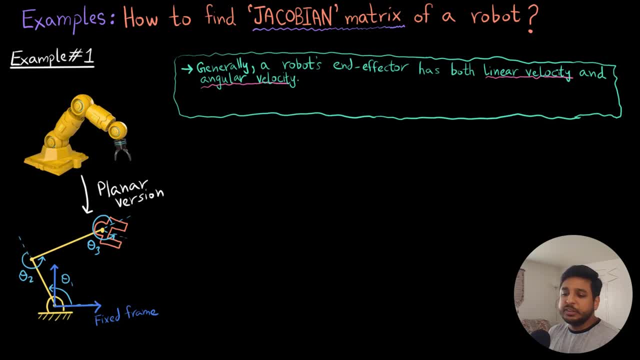 fast the robot rotates. and the second thing is that generally for a planar 2d robot such as this one right here, our jacobian is going to be a 3 cross 3 matrix. in some cases it can be a 2 cross 2 jacobian matrix. 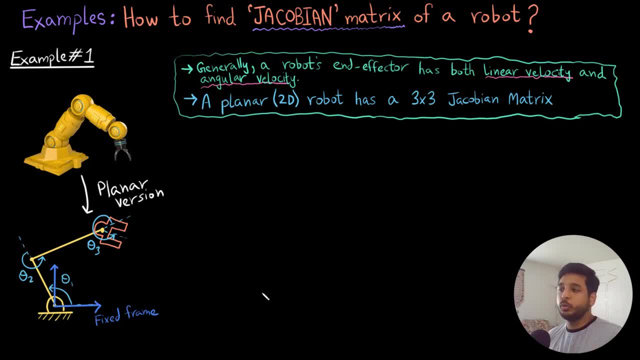 but that would be very rare. generally for a planar 2d robot it is always going to be a 3 cross 3 matrix. so the way we find out the jacobian is we first start out by doing the forward kinematics as Latitude histogram, like what we already know. that last one we are going to be doing here. 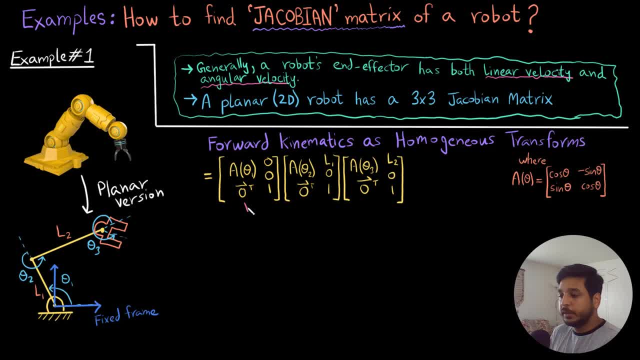 this is called a 3 cross 3 matrix, and there we have beenwith a window property of the radial component, and i would just like to add something to that: that what we take is negativeを and that uh, power, and this is not an wah, do that, this is yours, but this component of this, 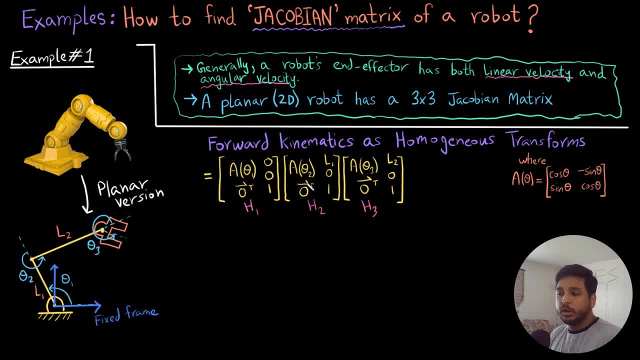 critical force. that is something that occurs when something has a needing of its Ahora, which is this one now moving forward. if i just multiply these three out, these three homogeneous transforms, i get this singular matrix right here. from this matrix, i already know that these two terms right here. they represent the position, the x and y coordinates of the end factor. so these 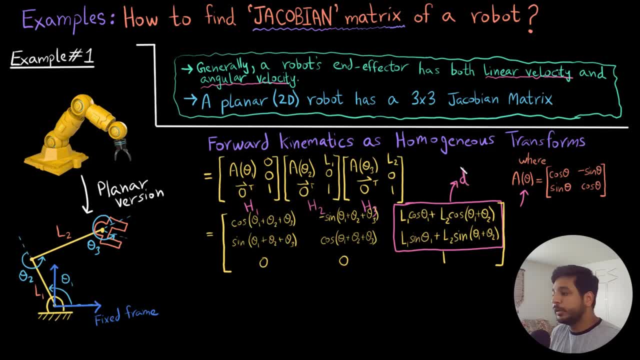 tell me the displacement vector, so i can call this d, which is just the x and y position of the end factor, and this theta 1, theta 2 and theta 3, which is common in all these four terms. what this tells me is it tells me the, the combined rotation of the end factor. so the combined rotation of the. 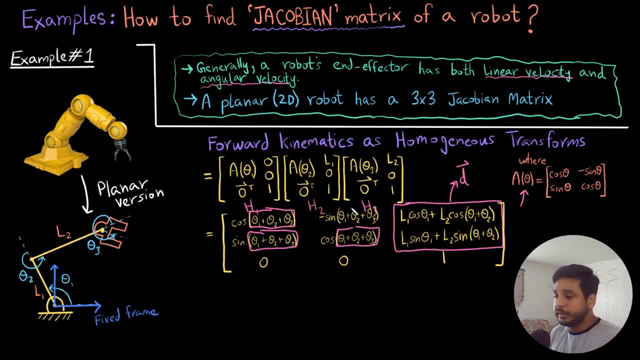 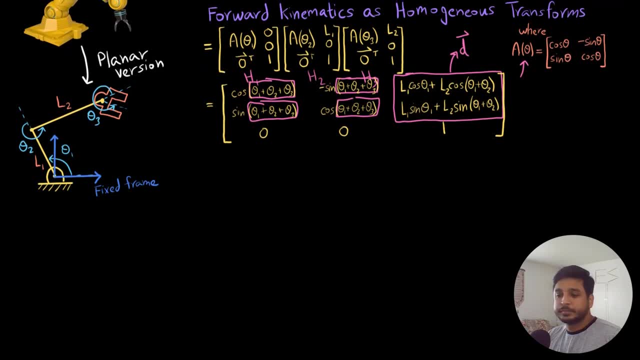 end factor would just be the sum of all the three thetas in this case. so moving forward, so i debate this- theta 1, theta 2 and theta 3 as phi and the displacement d is just this. i've just written it out in a slightly different form now in order to find the 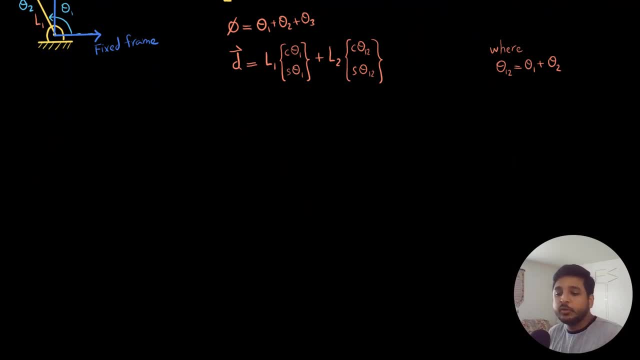 angular velocity and the linear velocity. so for angular velocity all i need to do is i need to take the derivative of phi with respect to time. so i differentiate it with respect to time. i get this: theta 1 dot plus theta 2 dot plus theta 3 dot. 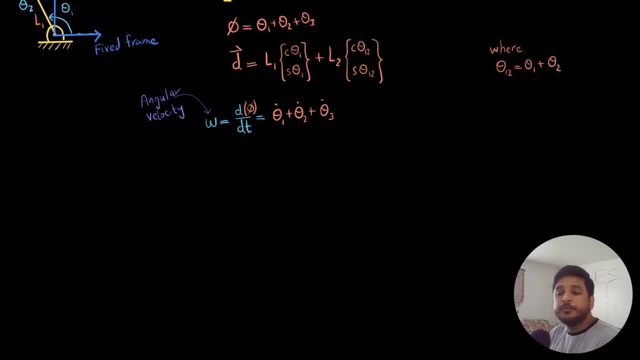 which is my angular velocity omega. and for the linear velocity i have to differentiate the displacement vector d with respect to time. so here i get the linear velocity and remember that all three thetas are a function of time. so if i go down now, all i have done is i have taken the displacement vector d and i have taken the displacement vector d. 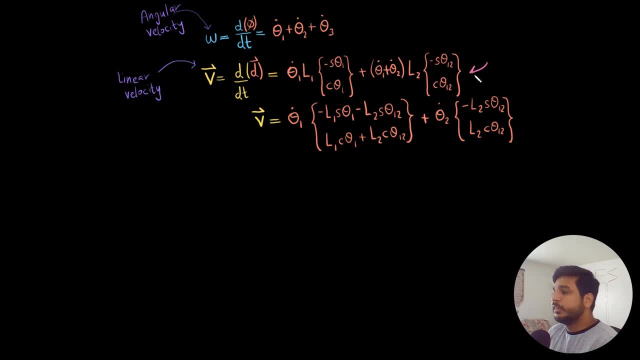 and i left the first one. i have taken the displacement vector d, splitting this into two resolutions. so if i put this integer in the following ways- so it's going to be equal to 1 comma theta times beta completion- i'm just going to multiply this thing to 2 comma theta by 1 and doing this I have fucking. 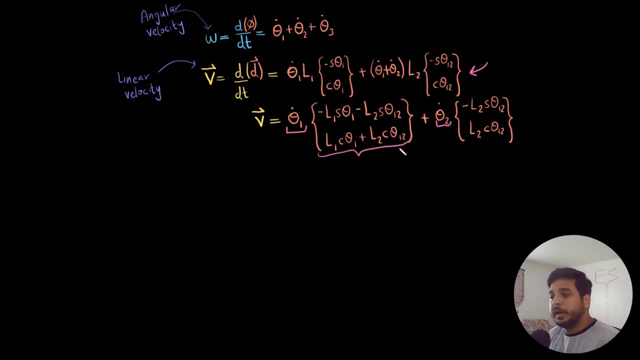 I think i probably have 1. so these are my two resolutions now what we actually have. so what we have to do is we have to multiply the sequential equations that go into theta 1 and theta 22 and the times two such things queued up in. 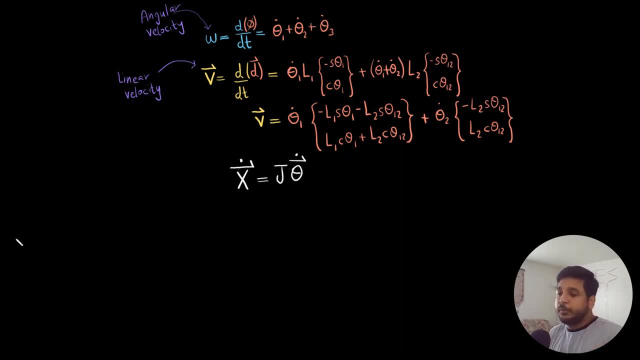 the whole plane of time. what do we see here is that theta 3 repository value is going to return to 1 έναまた. the simple way is that we make use of this equation, which is: X dot equals to Jacobian theta dot. so this equation just tells us how the Jacobian maps the joint. 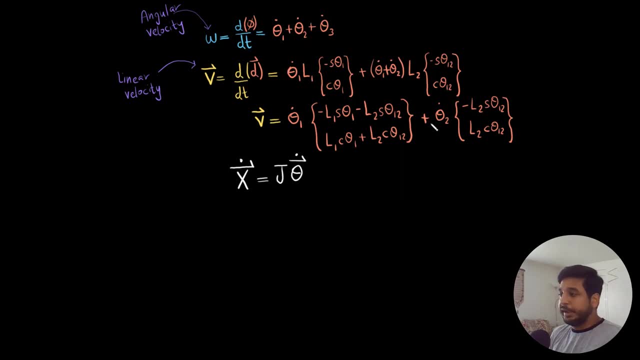 space to the end-effector space, and now we are going to be using these two equations in order to find the Jacobian. the way to do it is. I explain this so: X dot is just a velocity vector for the robot and we already know that the 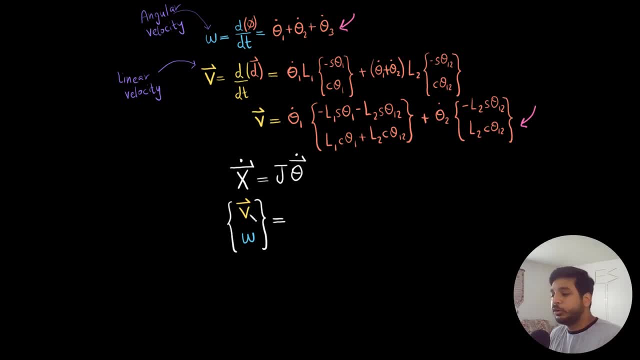 velocity is come, going to be comprised of both the linear velocity and the angular velocity. so this is the velocity linear velocity vector, this is the angular velocity, and then I just leave this space for the Jacobian and I write the vector of theta dots and using these two equations, this one and this one, I 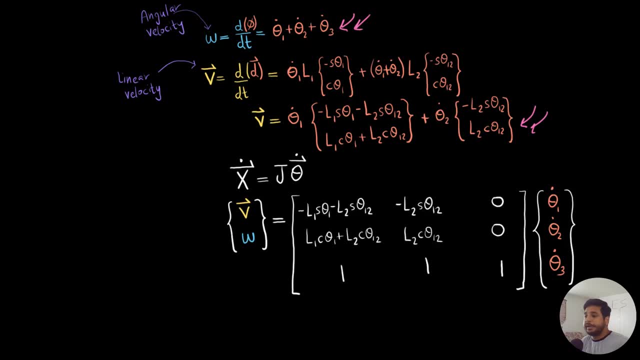 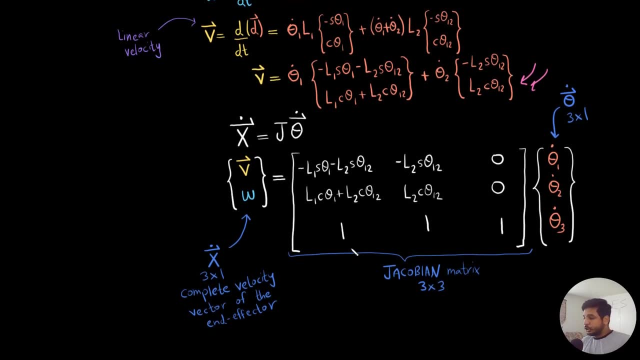 just fill out the Jacobian and I get this. so I know that this is my Jacobian, which is a 3 cross 3 matrix. this right here is my theta dot matrix, which is 3 cross 1 matrix. and this right here is again a 3. 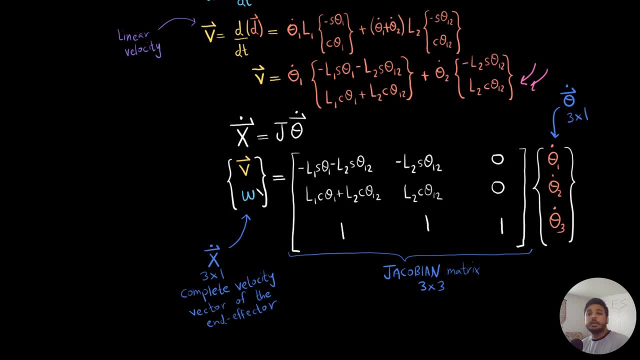 cross 1 matrix, which just tells me the complete velocity of the end-effector. so it is comprised of both the linear velocity and the angular velocity. and just like that, we have found out our Jacobian. Now, moving forward to another example, I would highly encourage you that you. 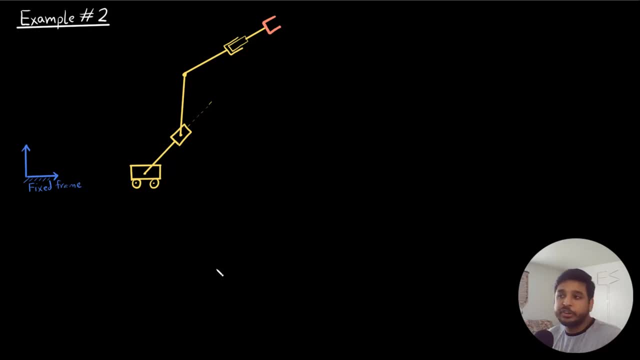 should give it a try, send the results to the public and, if you like this video, make sure to subscribe so that you can be notified every time I update a new video. Thank you and good luck, and see if you can find out the jacobian of this one. let me just tell you what is happening in this. 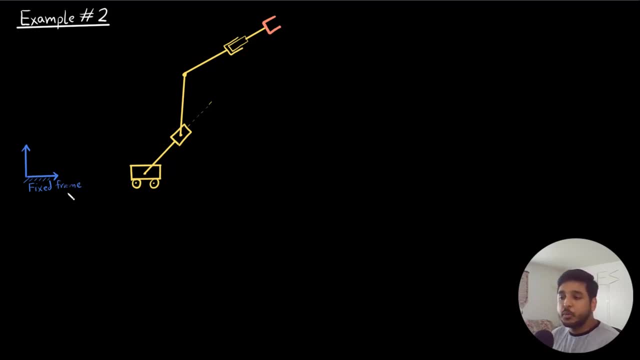 example. so i have, i have a fixed frame right here and i have a mobile robot which can move about in space and the mobile robot has a link here which is fixed at this point. so it is fixed here and this is a prismatic joint. what it means is that the length of this link- let me call this as 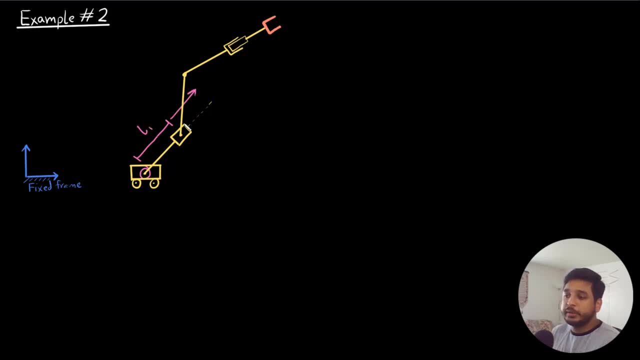 a one. it can increase or decrease in size, so this can increase or decrease in size. now, here again, it is a fixed joint, so it is not a revolute joint, it is a fixed joint. this one is a revolute joint and this again is a prismatic joint, so it can increase or decrease in length. let me just mark: 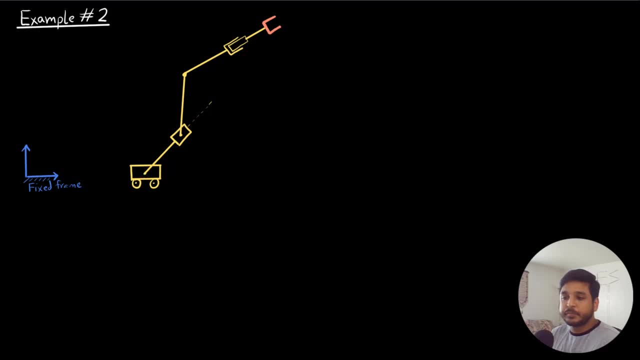 out what i have just told you. so here, this you instance, I am calling L0 and just for the sake of this example, I have kept it fixed, so you can think of it this way: that the robot is at a certain position in a space and we 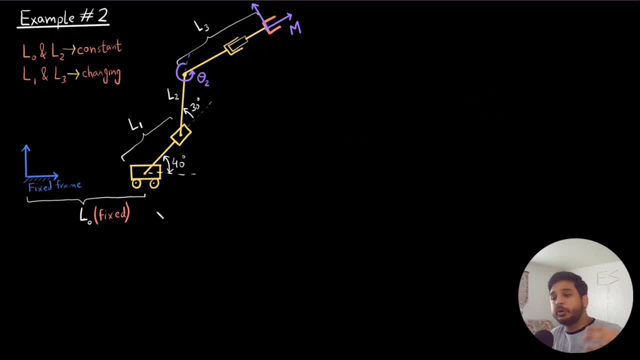 are just manipulating all the things and the robot remains stationary in a space, right? so L0 is fixed. L1, as we discussed, is a changing parameter. this angle is fixed, which is 40 degrees. this angle is fixed, 30 degrees. A2 is fixed. theta 2 is changing. A3 is changing. 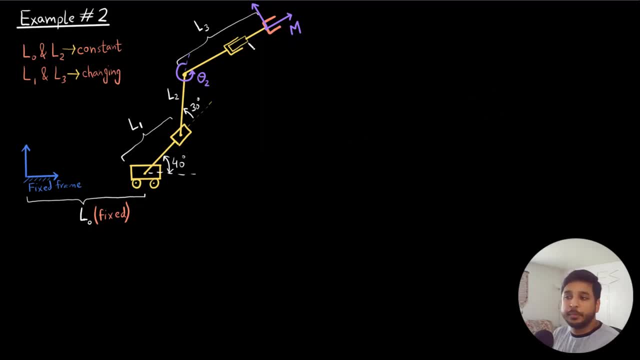 and here I have drawn the final frame, which is the moving frame. so A0 and A2 are constant and A1 and A3 are changing. now you can go ahead and give this example a try and see if you can find out the Jacobian of this one. I hope you did give it a try. 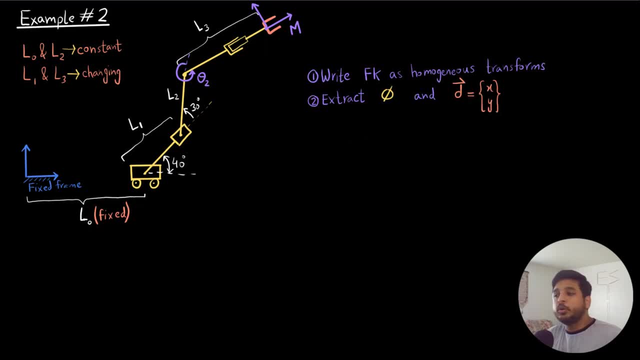 so the way to proceed with this is, first, you are going to write the forward kinematics as homogeneous transforms and secondly, you are going to extract the phi and the displacement vector from this. I am just writing out the displacement as being comprised of the x coordinate. 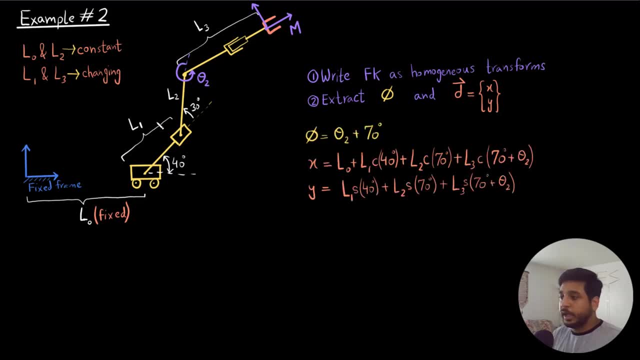 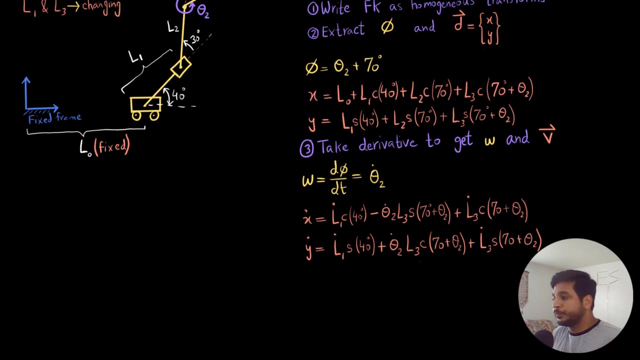 and the y coordinate. so if I do these steps, I get these three equations, which is phi is just theta 2 plus 70 degrees, and x and y are follows. now, in order to find the angular velocity, I just take the derivative of these with respect to time and I get the angular velocity and.